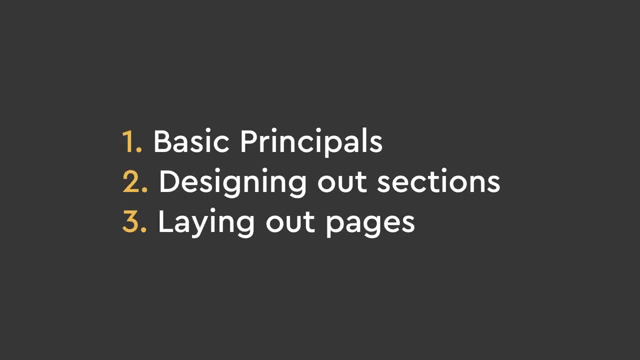 what makes a layout good versus bad. First we'll look at some basic principles of laying out a page, followed by laying out some sections to use, and then we'll actually pretend a client gave us some content and we have to lay out a website with it. With that being said, let's jump into the first. 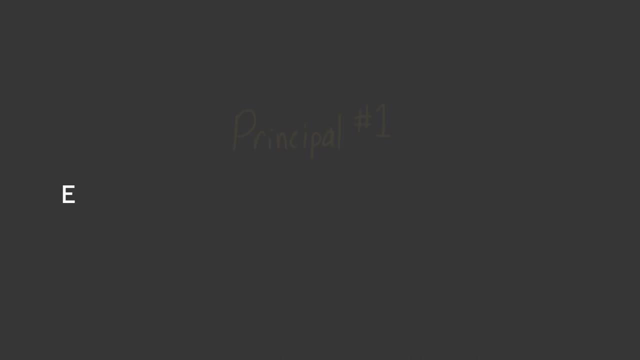 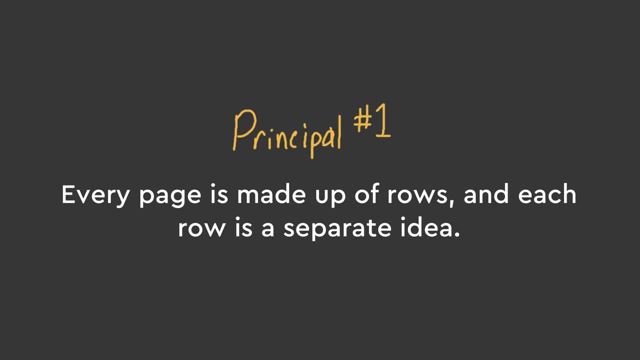 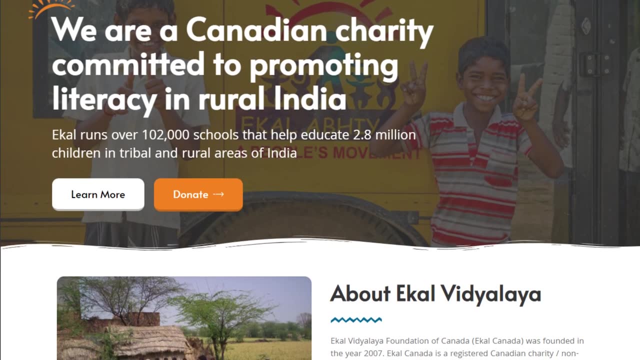 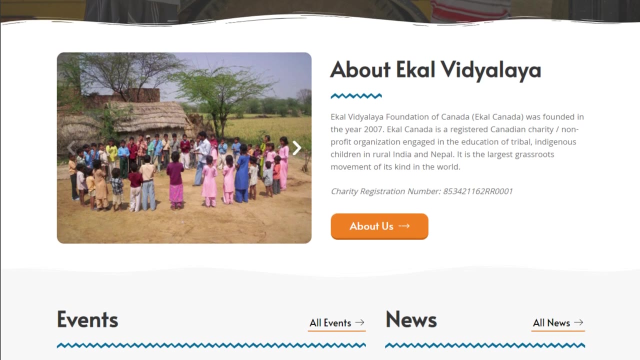 This simple principle personally made making website layouts so much easier to make and understand. I'll show you what I'm talking about. Check out this website. This is ecalca, a non-profit website I made. If you look at it in terms of rows, the layout becomes very clearly made up of smaller parts. 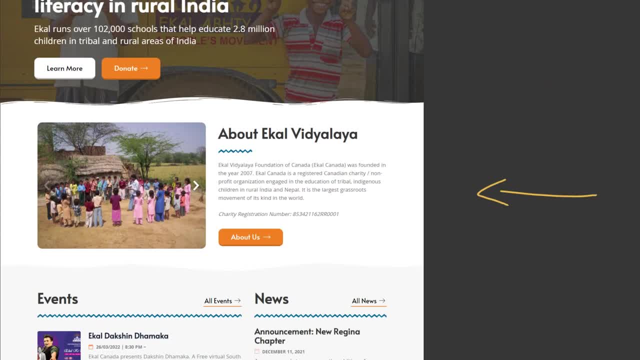 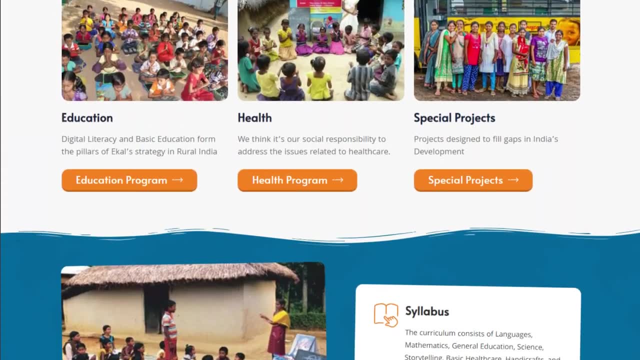 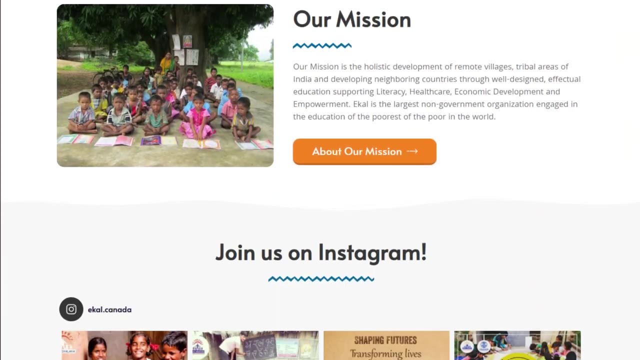 the rows There's distinctly a hero row, an about row, an events and news row, a stats row, and so on. Each row is a different idea pulled from the content, which means there should never be a single row that contains two different types of ideas in it. If you do, this will easily. 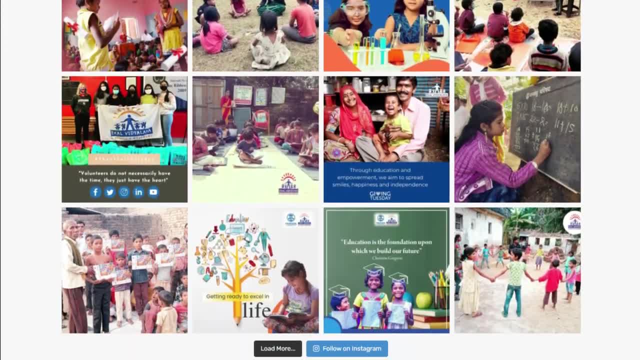 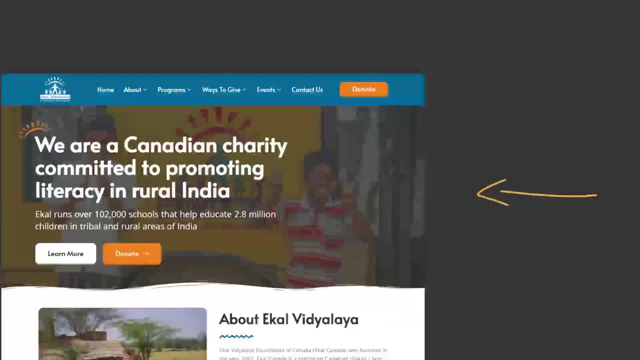 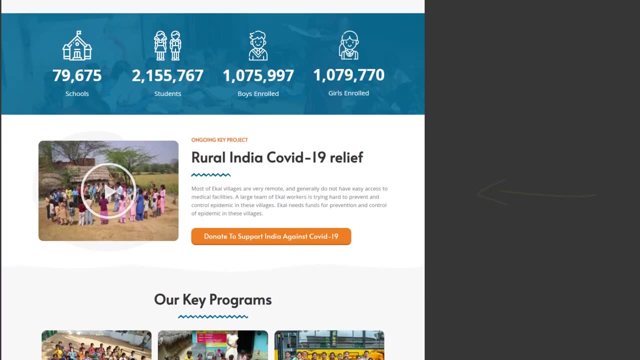 confuse the user and make for a poorer user experience. One thing that you may have noticed about the design is that each row is also made visually distinct. This one has a background image, this one has a white background, this one has a grey background, blue, white and so on. 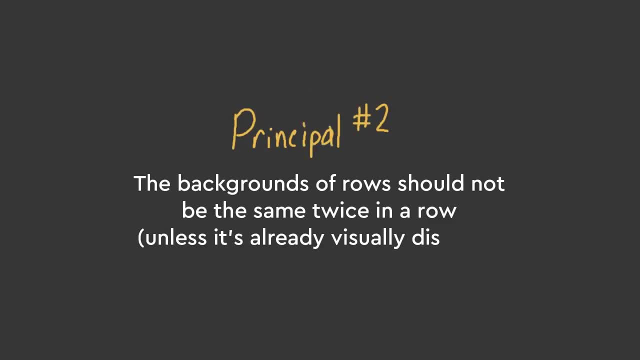 The background for these rows should never be the same twice in a row. If you do, the design won't look right and it will make for a poorer user experience. You can also have rows that have multiple rows inside them, like this, but this only. 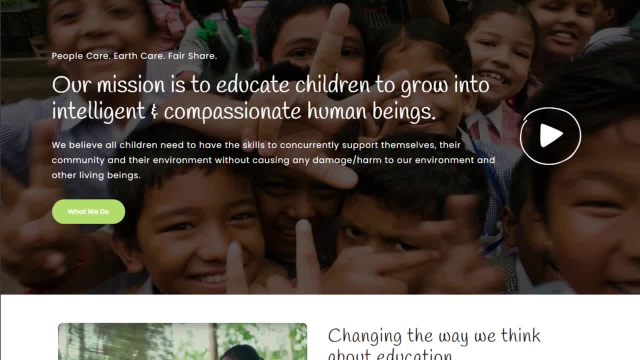 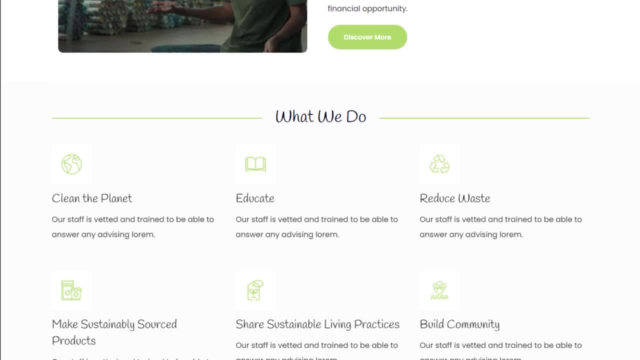 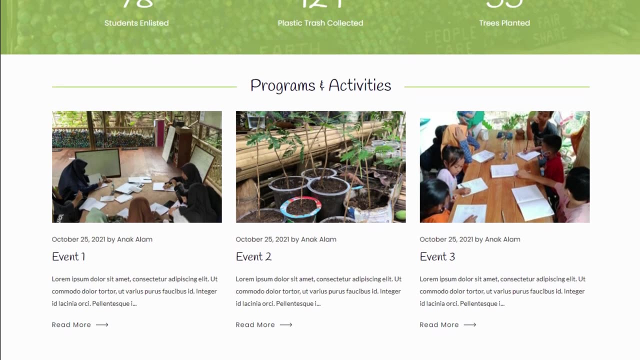 works if the content is related. It's not about separating the rows more, it's about separating the ideas. Now, if you're working on a website with a typical color scheme which is light colored rather than a dark mode style, Then you can get away with having a solid white color row and with a slight grey one. 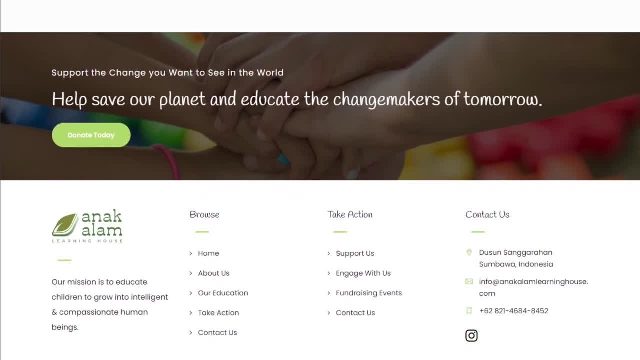 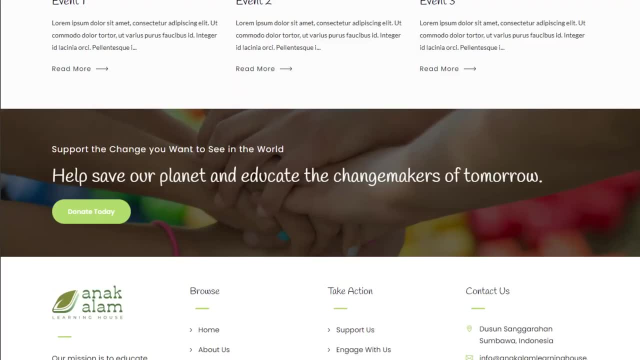 If it were dark mode, then you'd use a dark grey instead. I personally like to use the hex value F7, F7, F7 for my light grey, but it's up to you and your design. Then, of course, there are always background images you can use for rows. 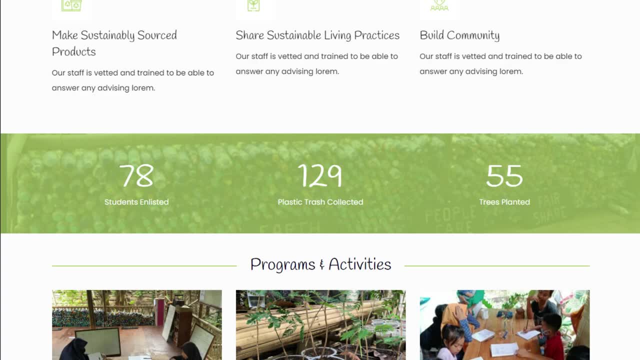 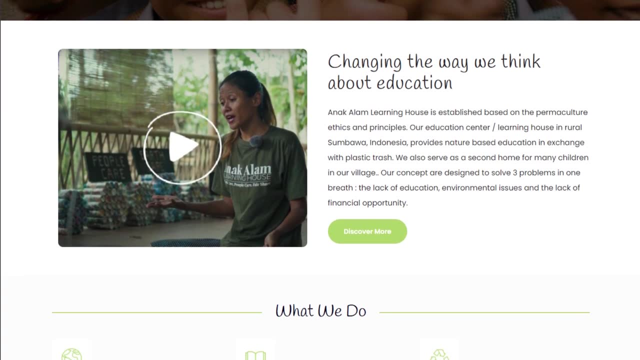 And, lastly, I like to use the primary colors of the website's color scheme for other rows as well. With just these different styles of rows, you're set to creating interesting, interesting and distinct looking rows. The idea here is to just make the sections visually distinct. You don't need to have 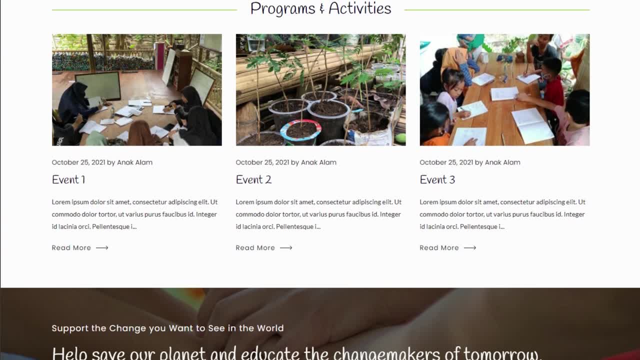 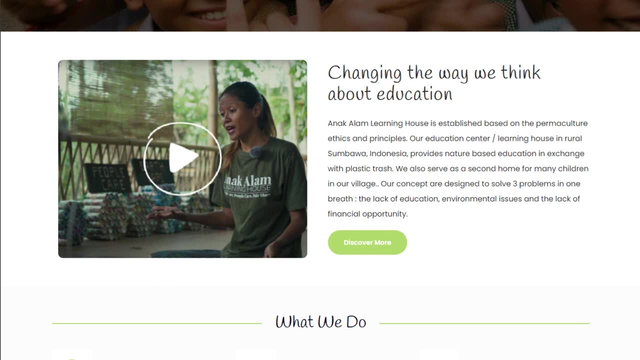 a different background style for each row, but as long as they're visually distinct and look separate in some way, then that's all you need. Another design related thing to keep in mind for rows is that each row should have some vertical padding on it. I use anywhere from 50 to 80 pixels for mine, but it's up to. 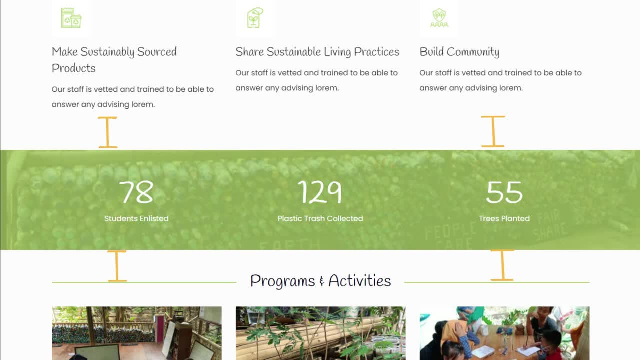 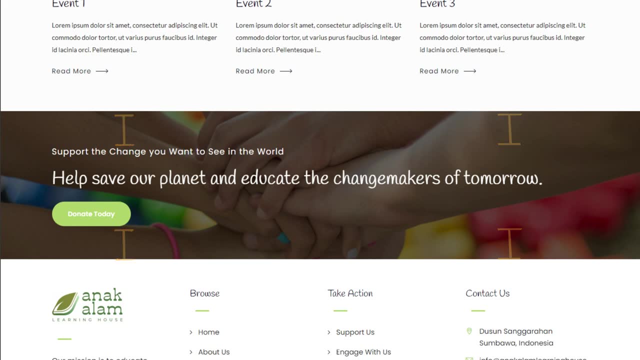 your design for the exact amount. Having this padding will make the layout look a whole lot cleaner and a whole lot more readable. It's important. I mention this because I see a lot of people not doing this or having way too little vertical padding. 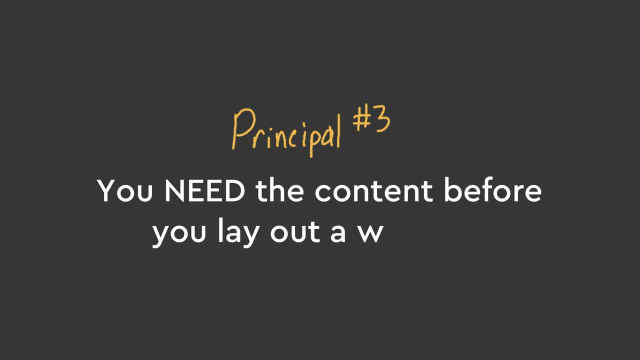 The last important thing you need to know about laying out a website is that you'll need the content first. If you want to make a layout good, you should never try to start with the layout and then later fit content into it. Instead, you should be taking the content and using the right. 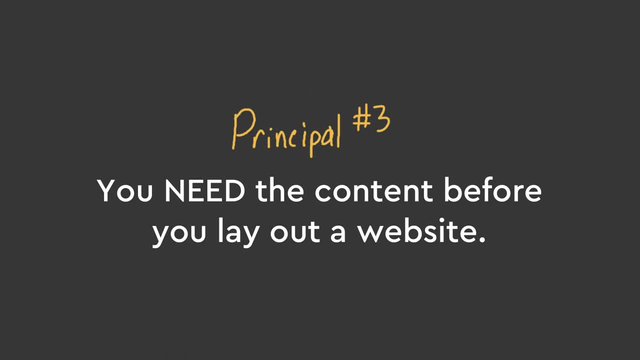 layout for that content. This is an important part to realize When designing a proper website. content should always come first, and the design should reflect that. Now, with those principles and guidelines out of the way, let's start creating some layouts and sections. 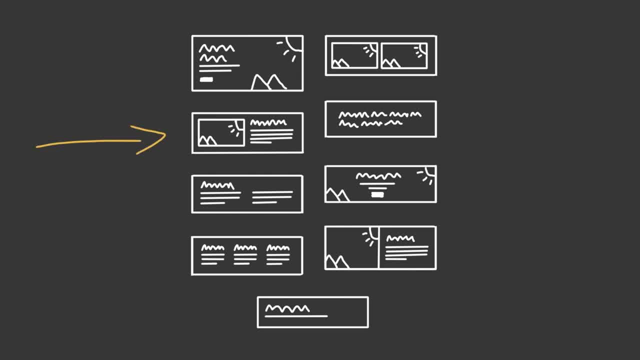 Here's a hero section: a. 2 column image in text. a 2 column text row. a. 3 column text row. a 2 column image row. a single column large text row. a call to action row, and these other two we'll talk about later. 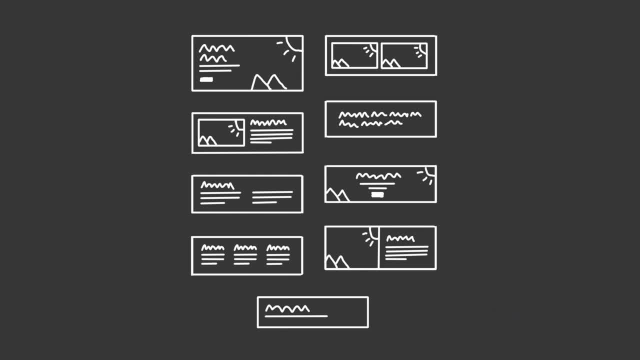 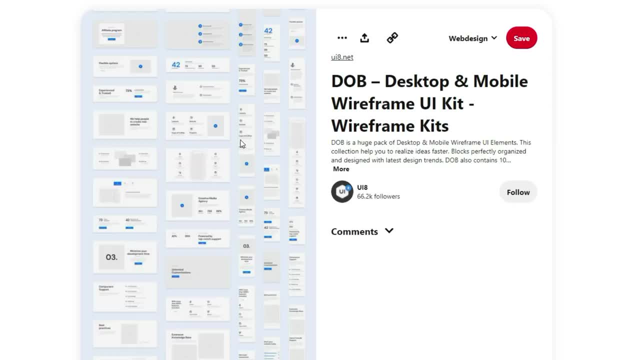 This is by no means all the layouts you can come up with, but this is just a few I'm going to lay out for this video. In fact, if you go to Pinterest and type in Web Design Page Blocks, you can find some more. that includes ones for testimonials and galleries. 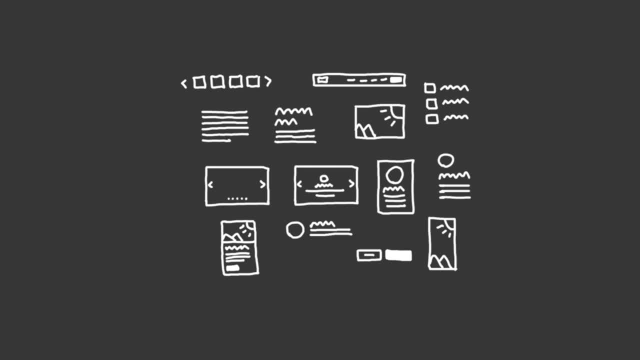 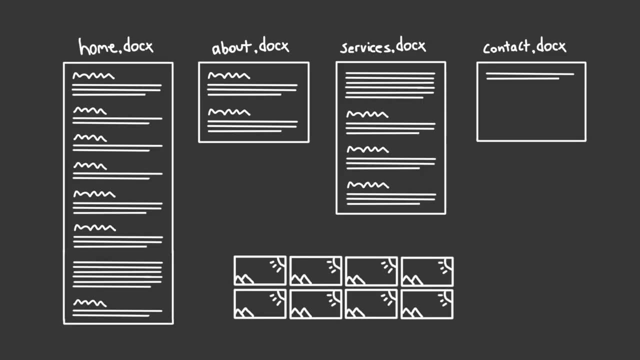 You could actually take this further by preparing some page elements too, but considering this video is more of a beginner level, I'm not going to go that in-depth Now. let's pretend our client gave us this content and let's start working with it. This. 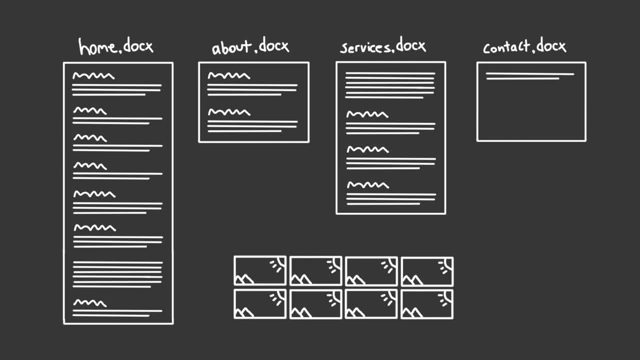 client of ours is probably some typical business like a lawyer, plumber or builder. We have the content for the home page, an about page, the service page and a contact page. We also have a dump of random images the client provided us to use throughout the website- Not every. 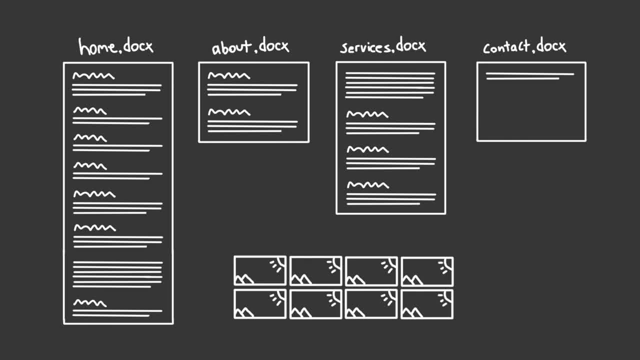 client will have documents laid out in such a way, but this is actually a typical way to see them outlined for the average brick and mortar business. Most of the time, you will be basically getting what you see from clients: A wall of text. 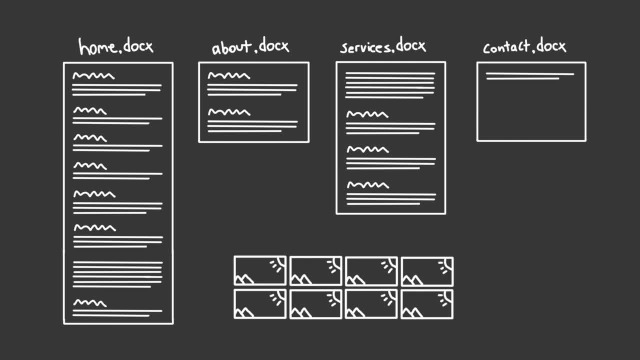 with some headings in between. I actually personally like this because it gives me full creative freedom to layout the content and use it in whatever way I want. Now that you have the content, it's up to you to determine what kind of layout works best with that content, provided Each part. 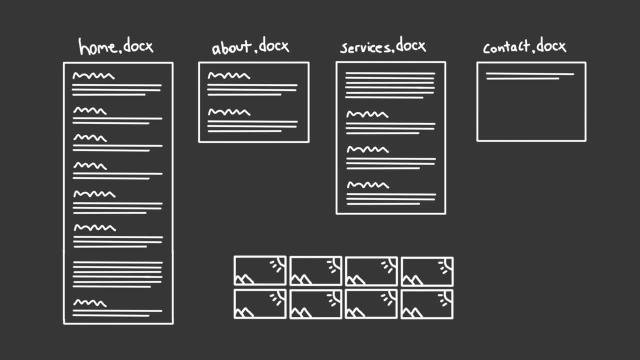 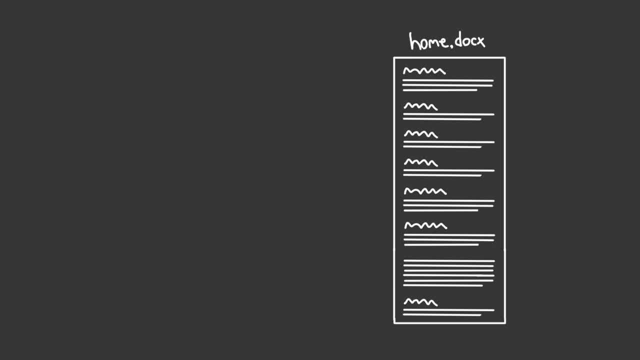 of the content will work better with a certain layout over another. Let's start with the home page. I already did a video on what I think the best home page layout should be supported by user experience, which I'll link in the description. but considering 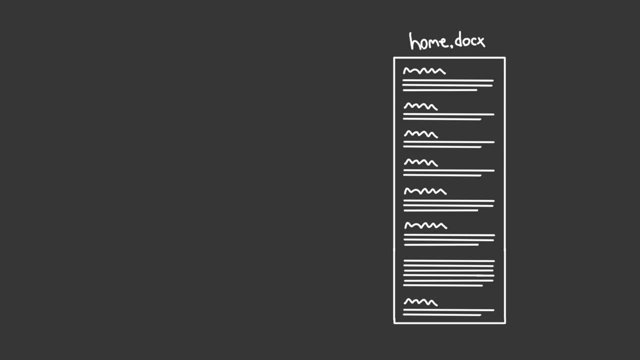 we have content here. we can make a new custom layout to reflect it. I know I said that the content would determine the layout, but there are also some web design trends that you should be following to create layouts familiar and that promote good user experience. 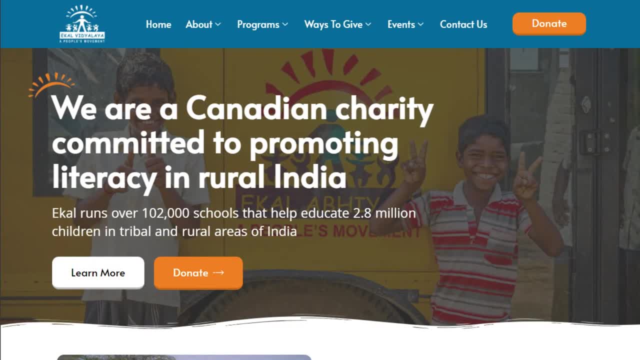 One of those trends is a hero section. This is the first row on the home page with a big background image, a heading, a paragraph and a button. I recommend this layout for 9 out of 10 home pages. It just works. It's informative, It's easy to use and it's 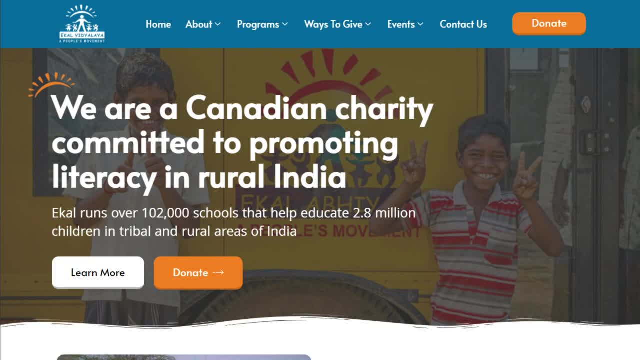 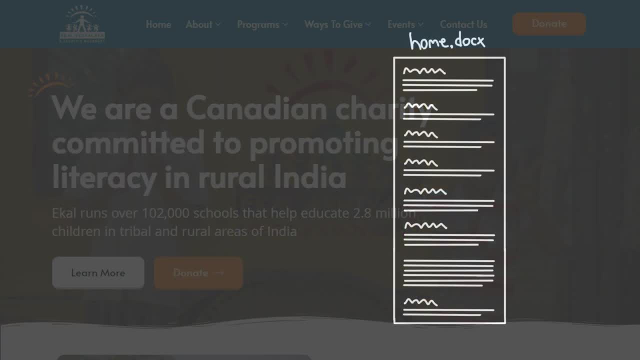 concise and gets clicks. It's also common, which means it's familiar, which is great for user experience. Now, just because the content we have here doesn't specifically outline content for the hero section, this doesn't mean you shouldn't make it 9 out of 10 times. this is actually. 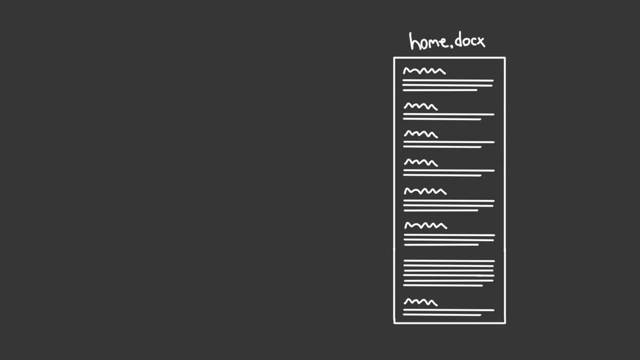 something I have to end up pulling from the other content to create. The typical hero section is just a heading paragraph and button, so it wouldn't be that hard to extract the content we need. So let's start with the hero section. 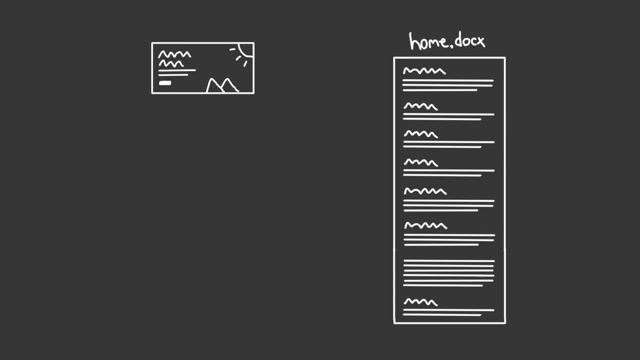 For the hero section row. we're of course, going to start with the background image style. I'll add in the row with the content inside it to complete it. And here's our first row done. Now let's look at the content again to see what kind of layout we should have next. 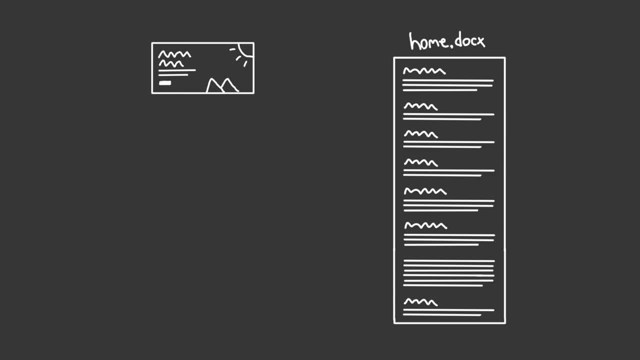 Now it should be pretty obvious what content in the document should be divided into rows. I can see right away. we can split up this section, this one, this, this, this and this And lastly this one. For our next section, it looks like we have a heading with a chunk of text. Let's browse. 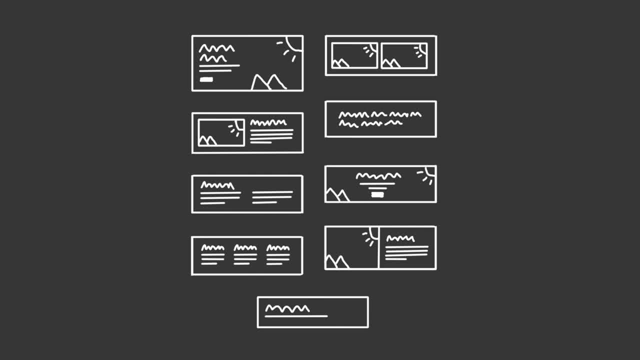 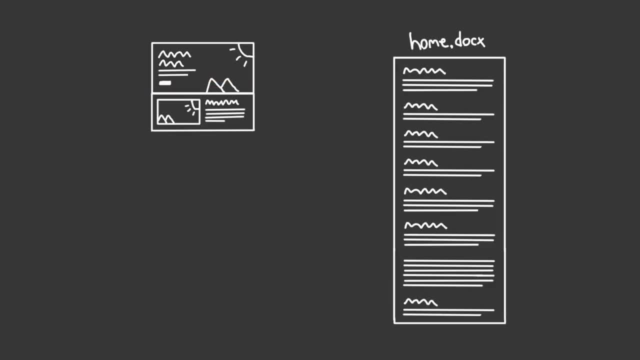 through our layouts to see which one would fit best. I think this one would fit best If we just paired it up with an image. we can use it for our second row. Another smaller rule to follow about laying out websites is that you should avoid walls of text. This: 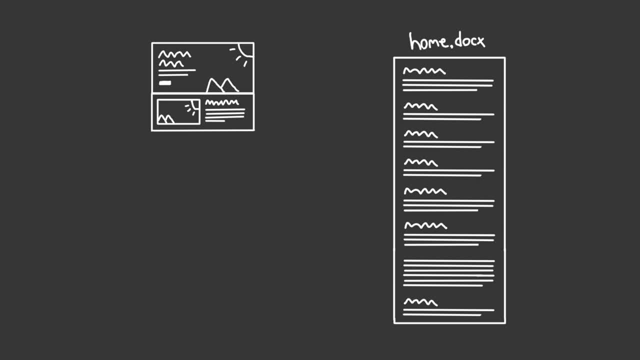 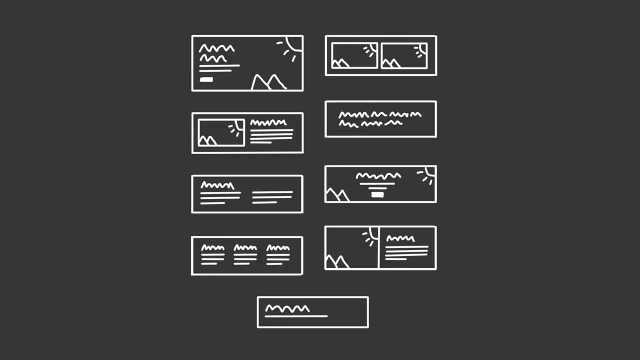 is why I chose the layout with an image: to avoid this. People tend to be quite visual, so I like to add in an image wherever I can, And images also add value to a page, so that's a bonus. Next up is these three sets of headings and paragraphs, The obvious choice for this layout. 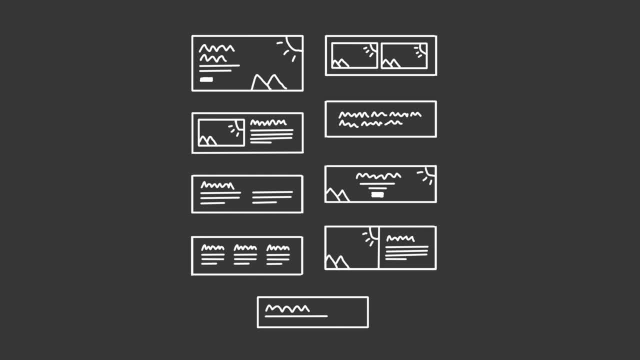 would be the three column layout. This one will work great. no images needed. However, there is a small problem with it. It just jumps straight into the content. Most sections should have some sort of heading to describe what the section is about And, based on the 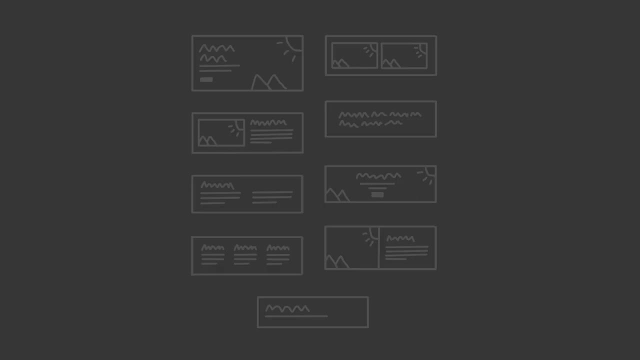 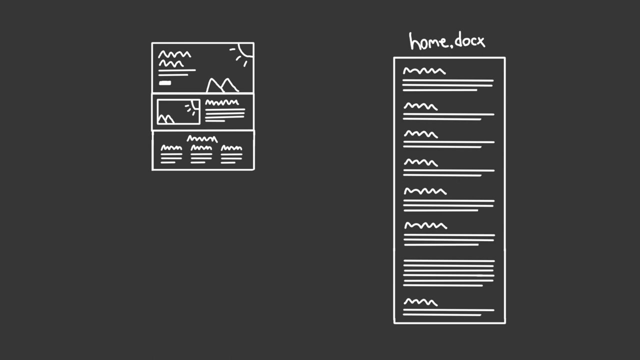 wireframe. we don't have this, so we'll have to add in a heading ourselves. There we go much better Now. this section's content can be easily scanned and has a purpose to it. For this row, I will also make it have the light grey background to differentiate it from the rows above and 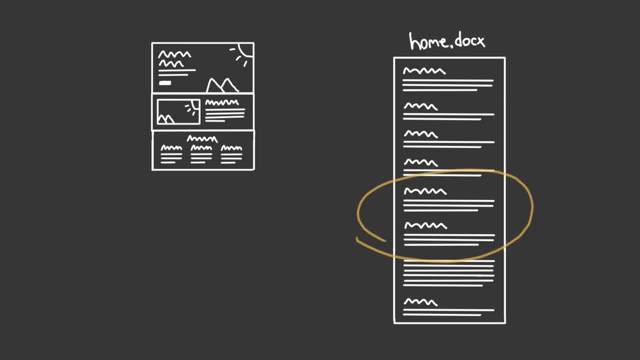 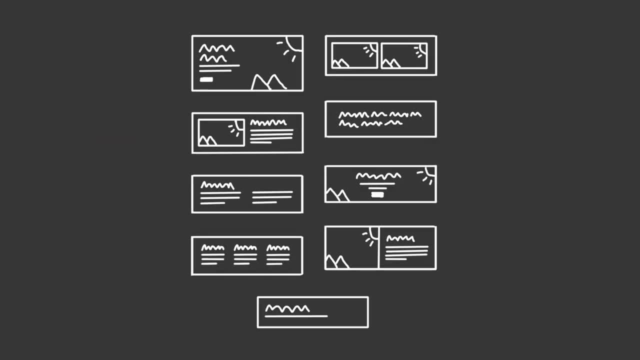 below it. Looking back at the content we'll actually add in these next two sections at once, The size of the paragraph seems ideal for another two column layout with an image and text, so we'll use that one again And again. we want to use images because they add more interest. 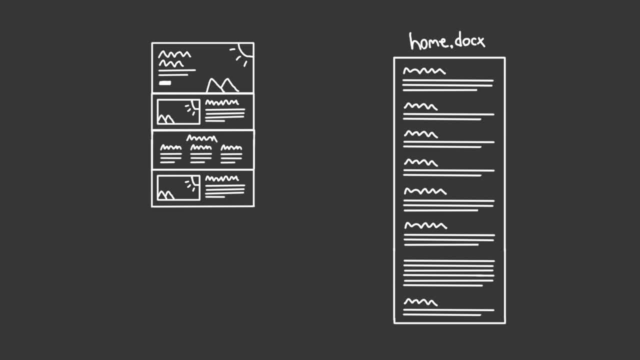 and value to the page. But because there's two of them, we can just swap the columns on the second row to mix it up and have a more interesting layout. Now for the background. I would keep them both white. I realize I'm looking at just. 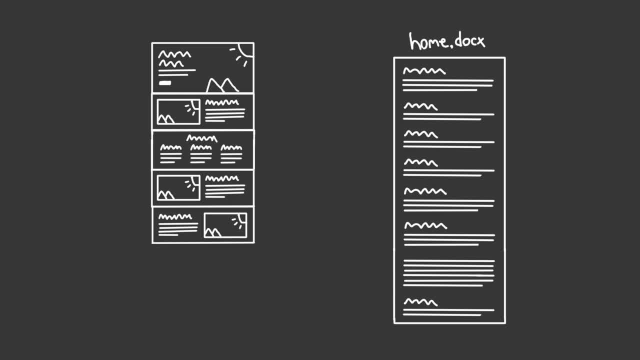 lines here, but I would imagine this content is related in some way. If you wanted to consider these two sections unrelated and therefore wanted to make them separate, you could use a layout like this. It's similar to the first one, but it uses a full width container, so the image spans the entire section and it will naturally look like this. Now for the background. I would keep them both white. I realize I'm looking at just lines here, but I would imagine this content is related in some way. If you wanted to consider these: two sections unrelated and therefore wanted to make them separate. you could use a layout like this. It's similar to the first one, but it uses a full width container, so the image spans the entire section and it will naturally look like this. 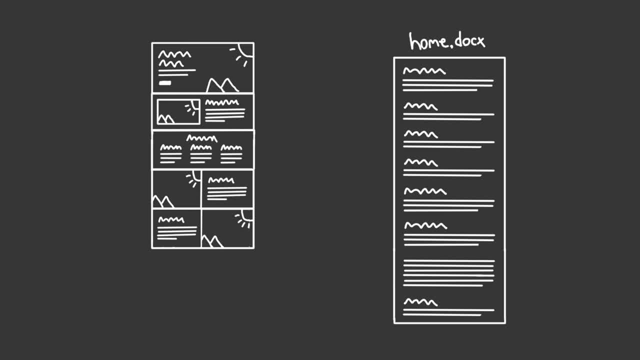 Next up is this basic wall of text. For this I will use a two column text layout. I'm not going to use an image for this one because we've already used images for the other ones and I think we could get away with just having text, Because it's a simple row. I also think 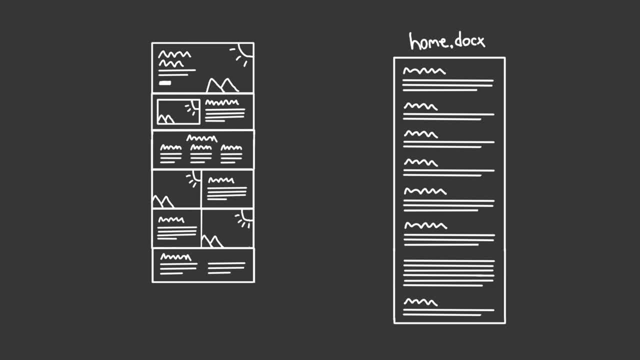 we can get away with having a solid color background. Back to the content. we can use this last little bit for a call to action. For this row, we'll use the content that we just created. For this row, we'll use the content that we just 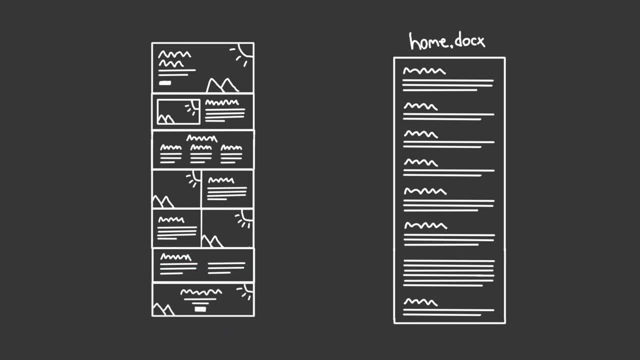 the image background. This works well for an absence of an image used for the row above, so there isn't an overwhelming amount of images going on. And there we have it. We use the home content to create a layout for the home page. Now, not every client will provide you with a lot of. 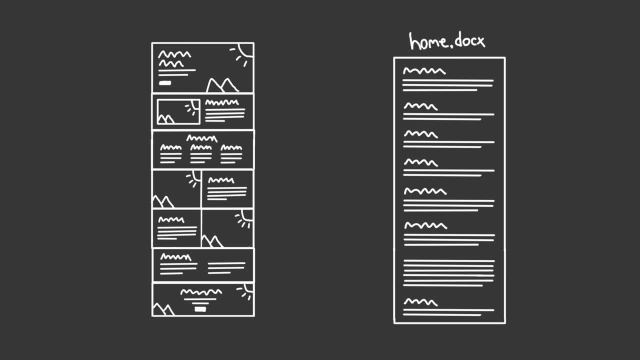 content for the home page, as my example client did. If they didn't, then it would be up to you to put some content together from the other pages, like the about page, to be able to build an effective home page layout. So that's the home page. Let's move on to the about page and see what. 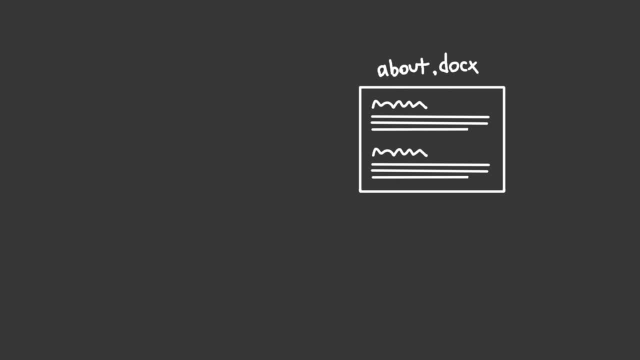 we can do In the effort to make this more realistic. when it comes to about pages, I find clients usually don't provide that much content. It's usually much easier for a client to talk about their services than it is themselves, which usually reflects in the content. So, to keep the theme, 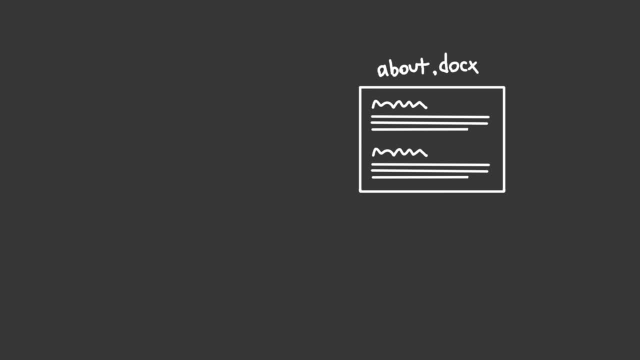 our about page content doesn't have much, just two paragraphs with headings. However, this is our first sub-page layout for the home page, So let's move on to the about page and see what we can do In the effort to make this more realistic. when it comes to about pages, I find clients usually don't provide. 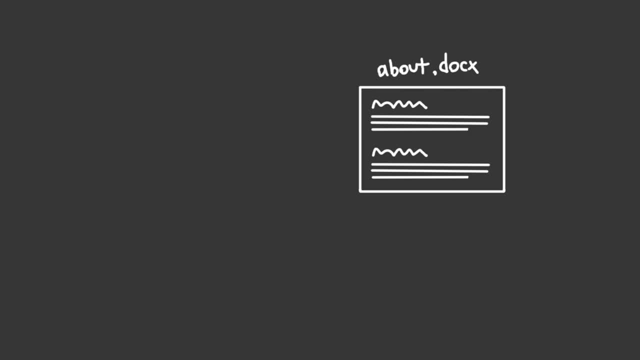 sub-page content. So let's move on to the about page and see what we can do. When I lay out sub-pages, I always find that there should be a consistent title section. In my opinion, for user experience, the title section on sub-pages should always be shorter than the height of the home page. hero. 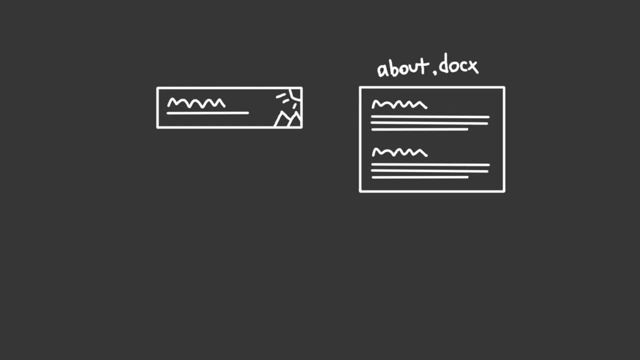 section. This subconsciously gives the user the impression that they are on a sub-page. just from this, which improves user experience. The title row should have the name of the page, possibly with a paragraph, and it should be a bit shorter than the height of the home page. hero section. 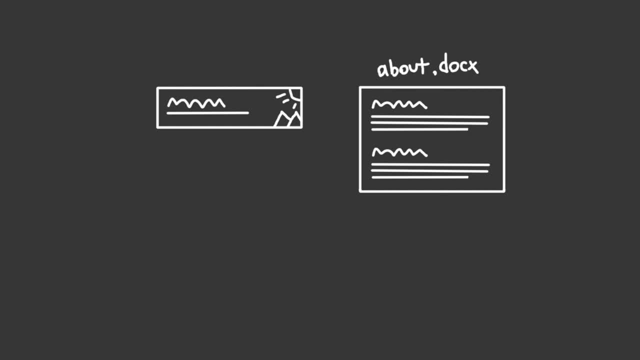 In the background image style row. I'll include the paragraph in the title row by extracting it from the content of the page. This paragraph should summarize what the entire page is about. It shouldn't be more than one to three sentences. Then for the content, I'll use an image in text. 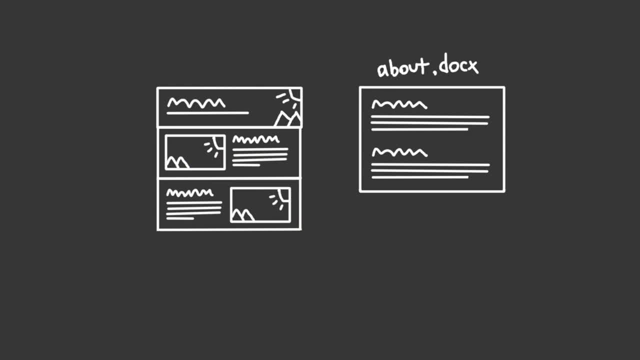 row, followed by another one, but swapped around again, Then what I like to do on sub-pages is create a call to action section at the bottom to help for conversions. Considering there's already one on the home page, I could just copy and paste this for this page. 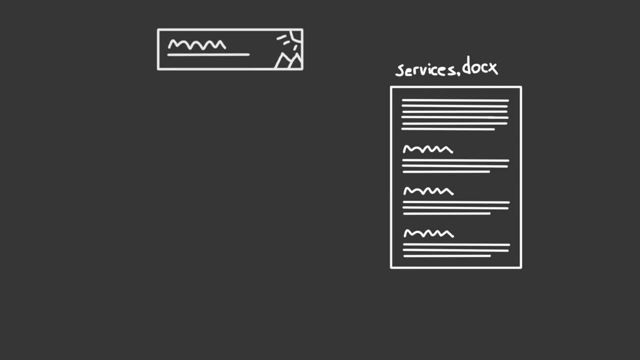 Next for the surface page: First the same title section as the about page and then, looking at the content, we have one large paragraph to deal with. next, Now that this paragraph appears a bit bigger than the previous ones we worked with, I don't think the two column image in text layout will. 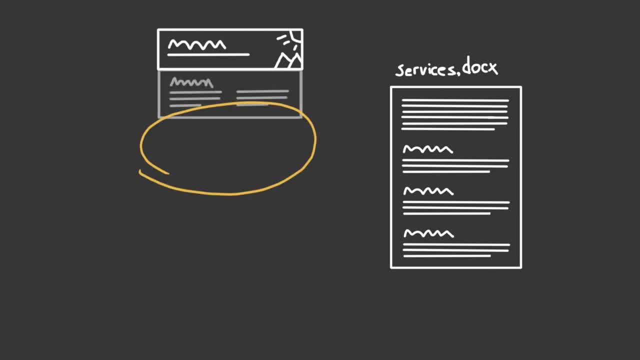 work. Instead, we'll use the basic two column text layout. Once again, the content didn't appear to have a heading, so I'll have to add in one of my own For this layout. I'll include it above both of the paragraphs. 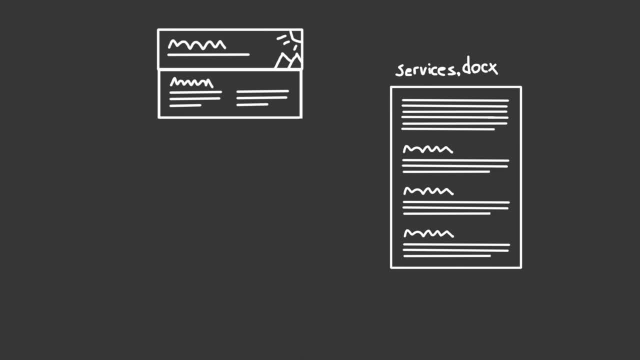 Next is what probably would be the content for the individual surfaces. I will use the layout we mentioned before for this one: the full width image and text layout. There's three sets of content for this one in the doc, so we can alternate the layouts so it looks more interesting. Finally, I will end the page with another. 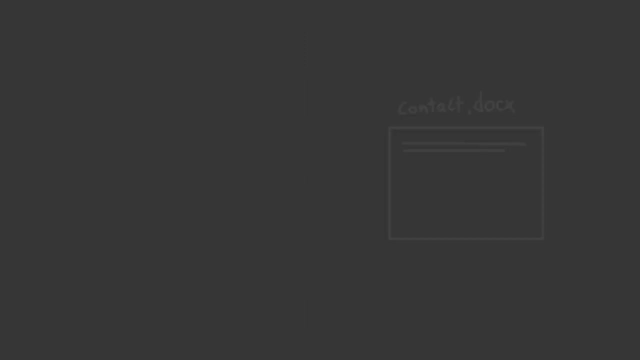